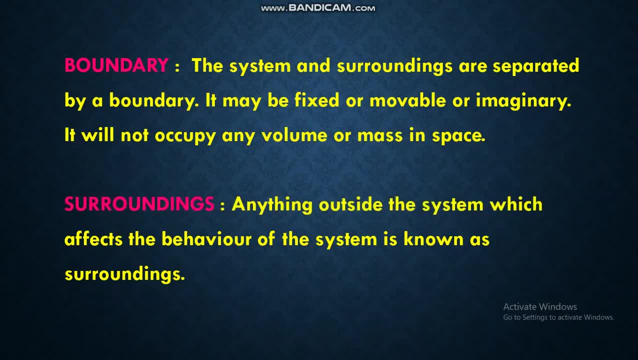 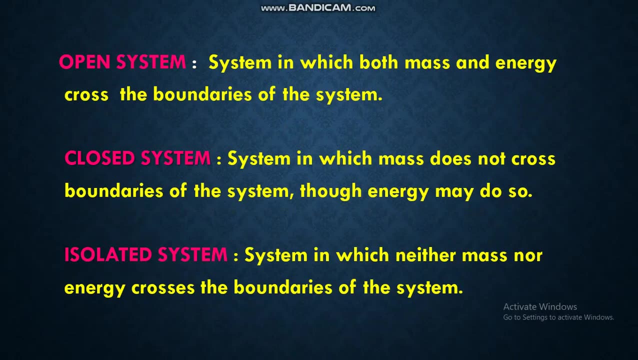 volume or mass in space. So next one is surroundings. Anything outside the system which affects the behavior of the system is known as surroundings. Next one system is divided into three types: open system, isolated system. First we see open system System in which both mass and energy cross the boundaries of the system. that 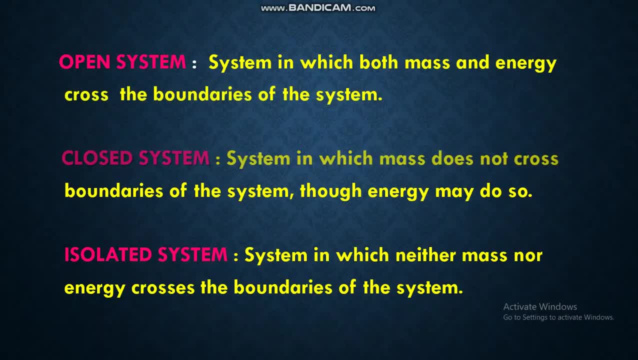 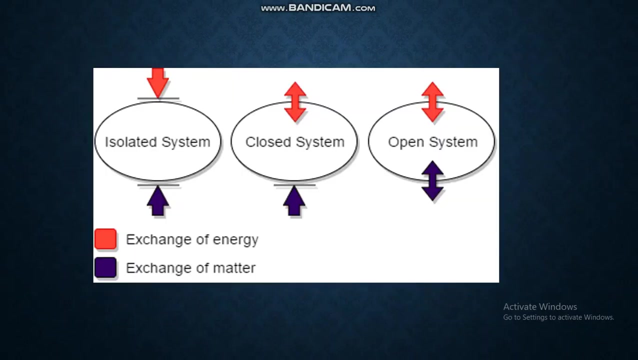 is open system, Closer system, System in which mass does not cross boundaries of the system but energy will cross the boundaries. Isolated system, System in which neither mass nor energy cross the boundaries of the system. So we can see in a simple diagram. So you can see open system in which exchange. 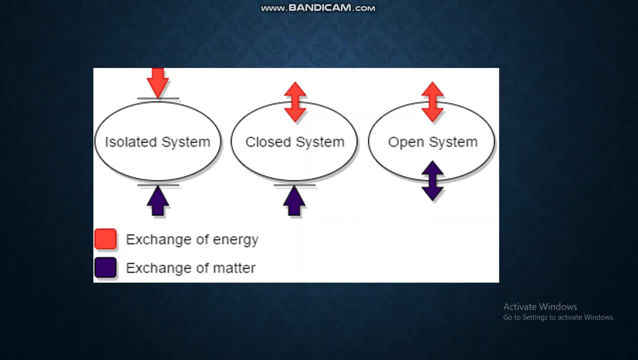 of energy and exchange of matter. both takes place. So: closed system: only exchange of energy takes place, no exchange of matter. Isolated system: no exchange of energy, no exchange of matter. So in this way we can easily understand the three systems. Next, 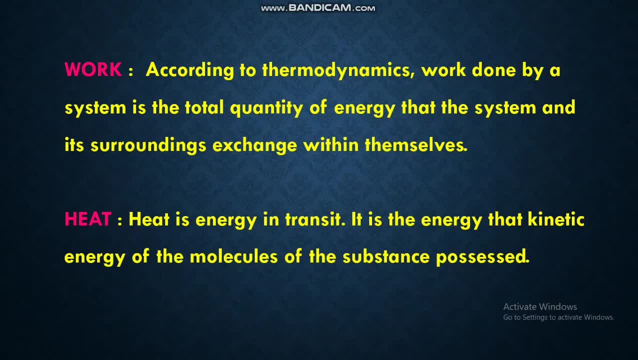 definition is work. So, according to thermodynamics, work done by a system is the total quantity of energy that the system and its surroundings exchange within themselves. Next definition is heat. Heat is energy in transit. It is the energy which the kinetic energy of the molecules. 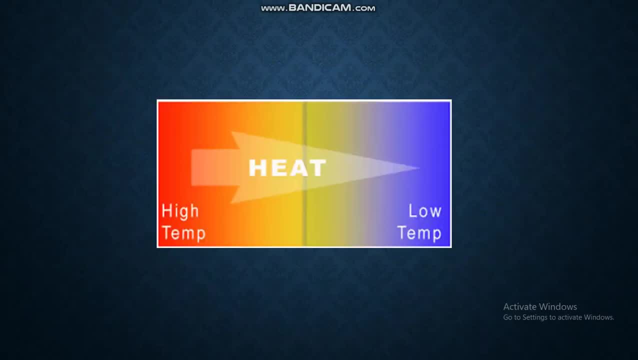 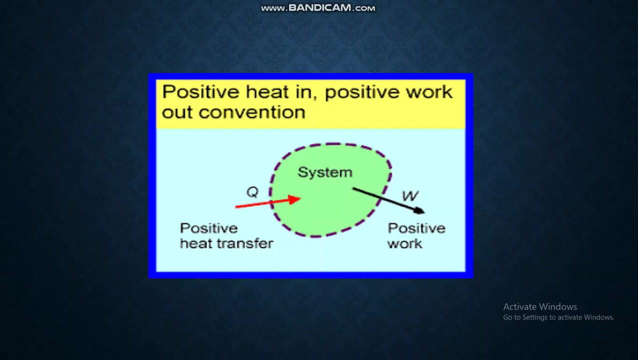 of the substance possessed. So you can see heat. Heat basically transfers from high temperature to low temperature. So, similarly, any system we can see how the heat transfer as well as work- both will be happening- can see positive heat transfer. Similarly, how is the work is exchanged between the system and 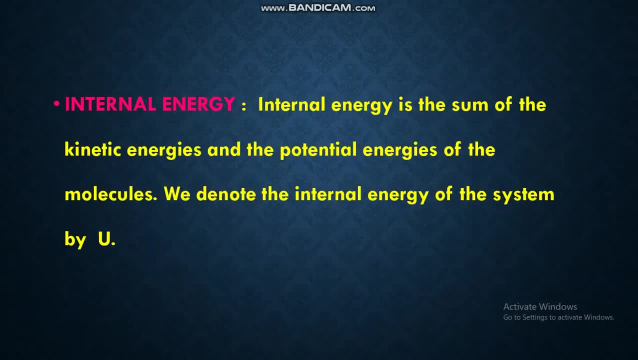 surroundings. Next one is internal energy. Internal energy is the sum of the kinetic energies and the potential energies of the molecules. So we denote the internal energy of the system by the symbol U. So this internal energy is very important in this chemical engineering thermodynamics.